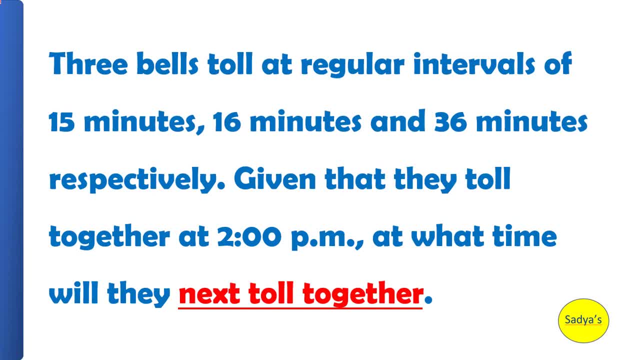 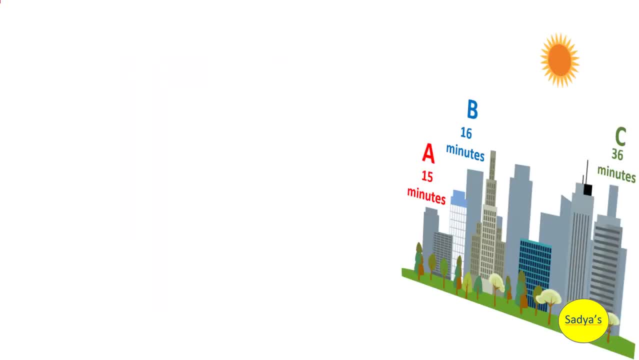 Next told together. This indicates repetitions or next occurrence, and we find it using LCM. So let's find the LCM of 15,, 16 and 36, which will tell us exactly after how many minutes the three bells will tol together. again, There is no common prime factor of 15, 16 and 36. 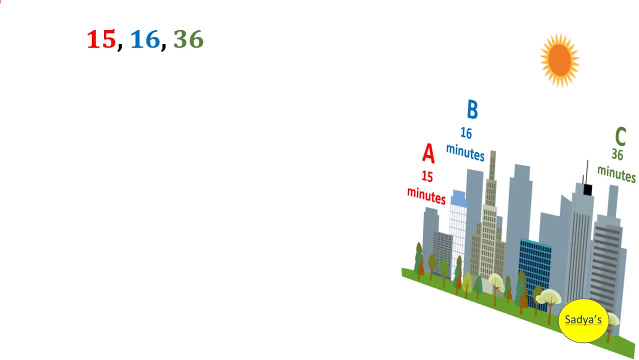 so we start dividing by uncommon prime factors. Since 2 is a factor of both 16 and 36,, we divide by 2.. 15 remains as it is. 16, divided by 2 is 16.. So let's find the LCM of 15,, 16 and 36.. Since 2 is a factor of both 16 and 36, we 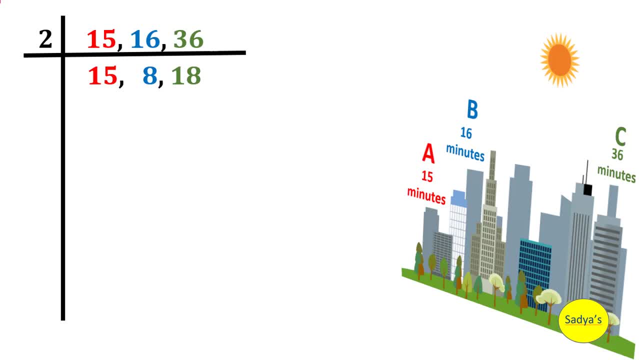 2 is 8 and 36 divided by 2 is 18.. Again, 8 and 18 are divisible by 2, so we divide them by 2.. 15 remains as it is. 8 divided by 2 is 4 and 18 divided by 2 is 9.. 4 is still. 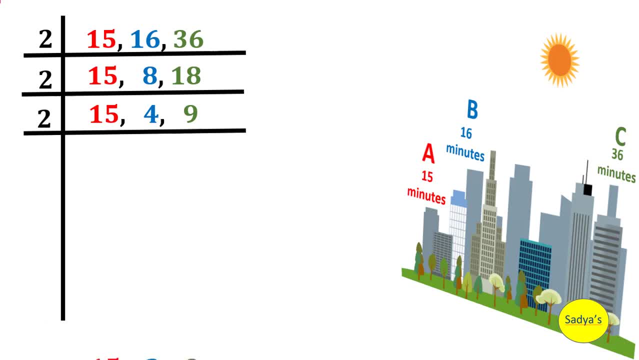 divisible by 2. so we divide 8 by 2.. 15 remains as it is: 4 divided by 2 is 2 and 9 remains as it is Dividing 2 by 2. we got 1 in the center and 15 and 9 remain as it is: 15 and. 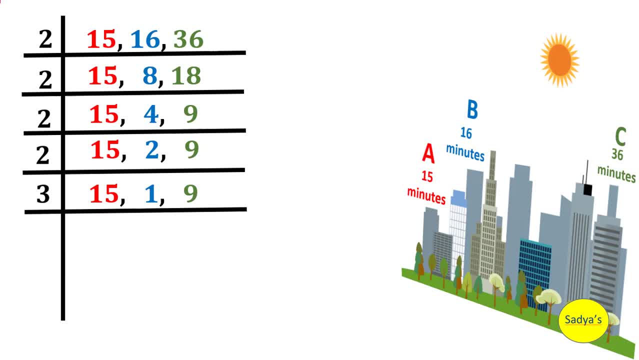 9. both are multiples of 3.. So dividing them by 3 give 5 and 3.. Again, dividing 3 by 3, 5 remains as it is, 1 remains as it is and 3 divided by 3 gives us 1.. And lastly, 5 divided. 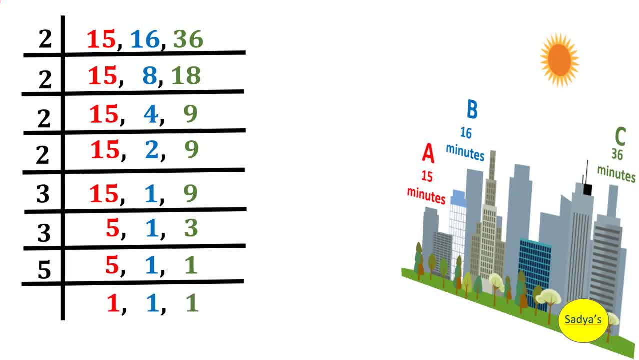 by 5 gives us 1.. So we have got 1's in the remainder And LCM is the product of all incorrect answers. Anav: competent: the numbers written on the left. So the LCM is 720 minutes. This LCM means that the 3. 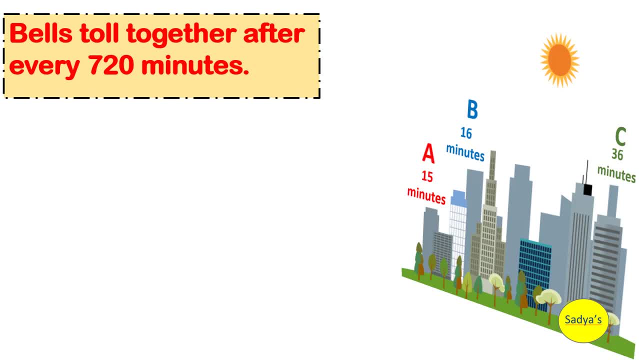 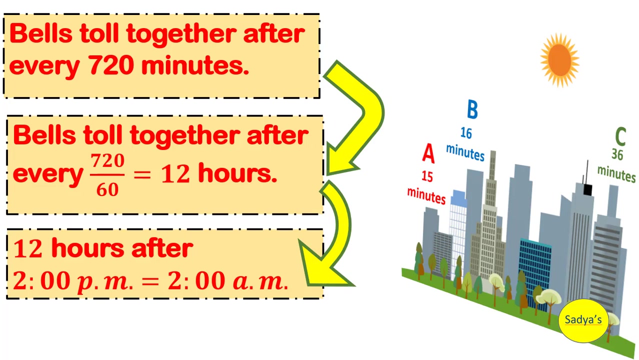 bells toll together after every 720 minutes And we know to convert minutes into hours we divide by 60. So 720 divided by 60 gives us 12 hours. So after every 12 hours the 3 bells toll together. As stated in the question, the bells had sounded together at 2.00 pm.